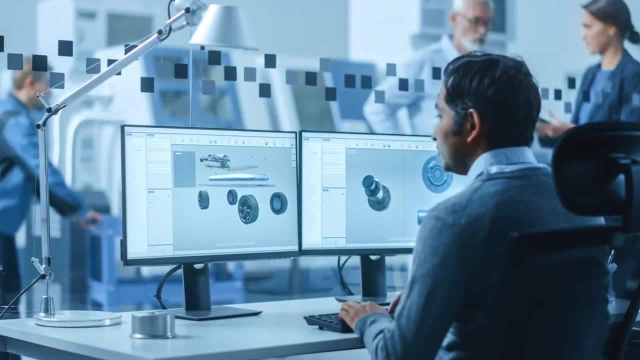 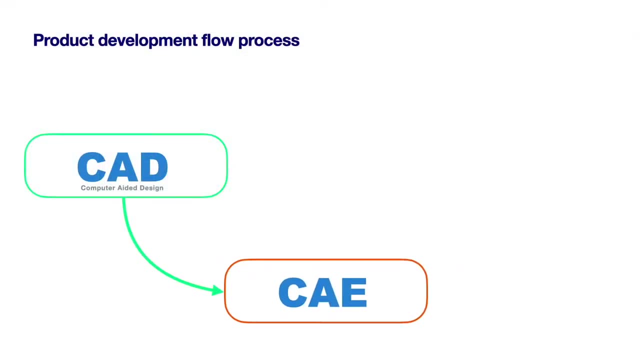 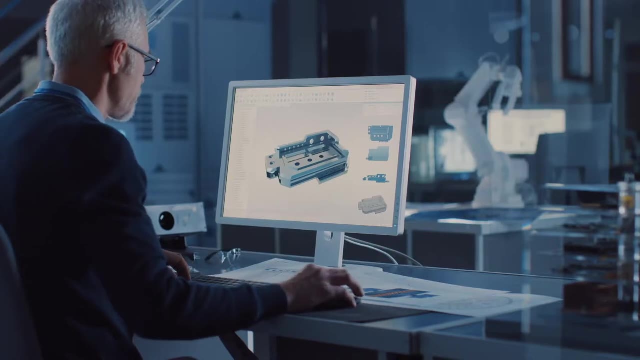 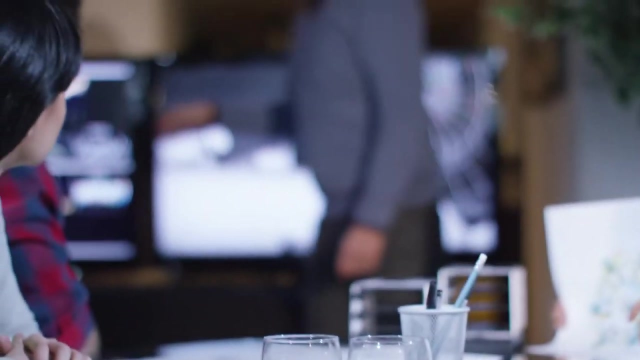 a product. After that, after designing, after finalizing a design, it will enter into one more phase, That is, CAE, computer aided engineering. In this phase we can call it as R&D phase, research and development phase. So in this phase an engineer is going to suggest a design or design. 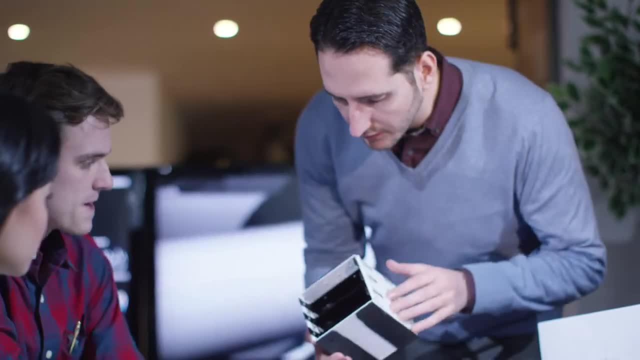 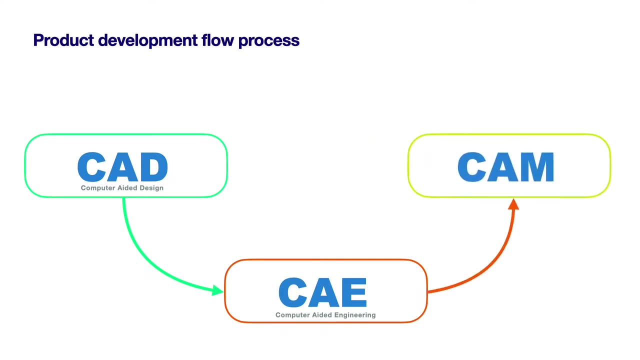 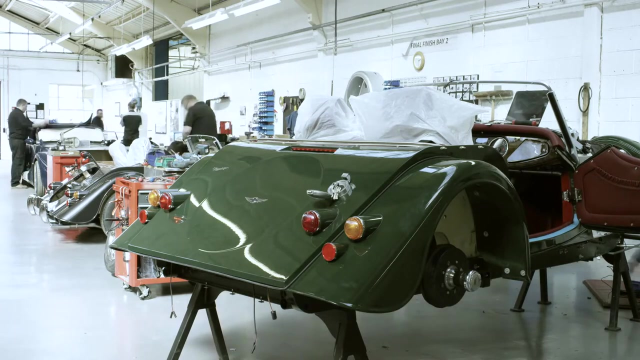 change. or we can say he is going to validate a design. After validating a design, it enters into CAM phase. So this is the computer aided manufacturing phase And in this phase we are, our industry is going to finalize a product and there a mass manufacturing will happen and this product- 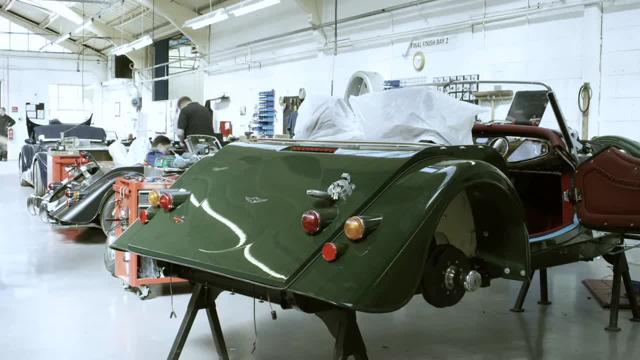 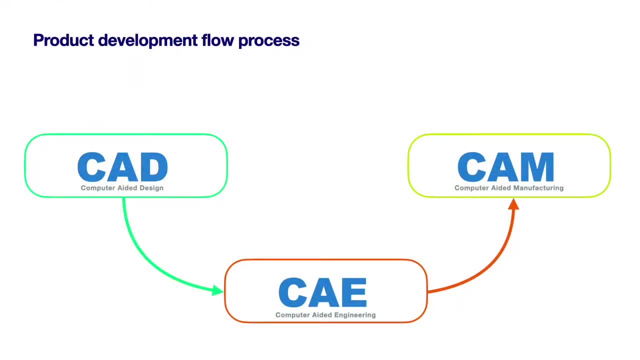 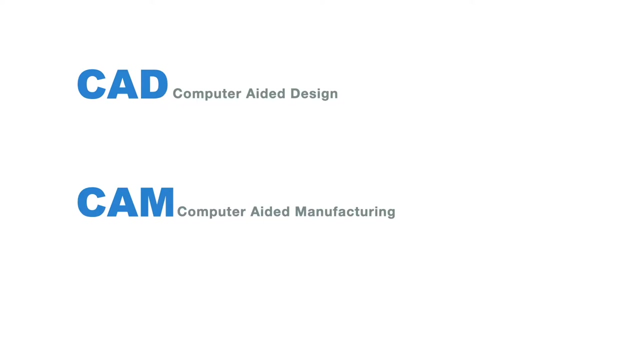 will reach to the customer. So this is the process, how a product will be developed in an industry. Okay, So in this phases, very popular phases or very known phases within common people, is CAD and CAM, computer aided design and computer aided manufacturing. 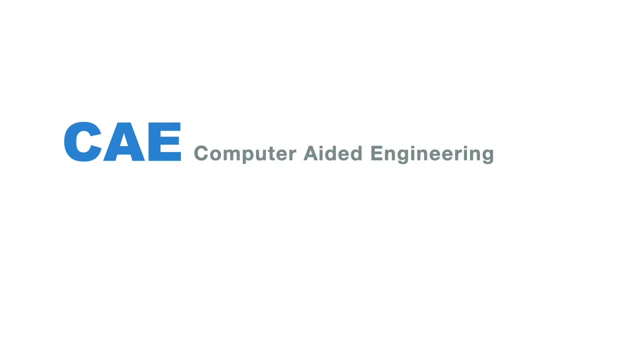 But this CAE process, or CAE phase, is a hidden phase and it is an R&D phase which is not familiar within many people. So hence we are going to discuss about this phase, both FEA or CAE, both phases are same phases. 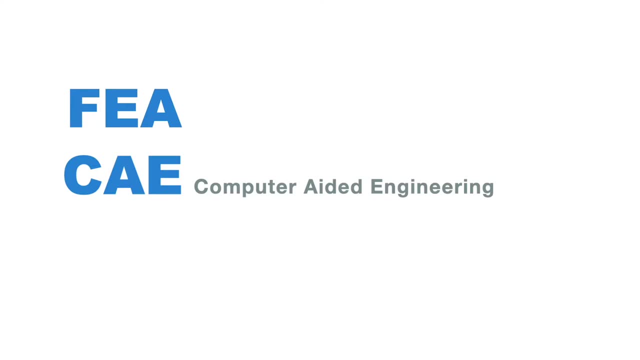 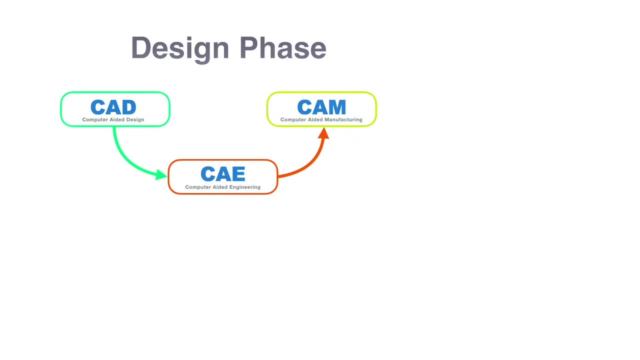 gong tá 钟, mỹ tá gi 승 case. conreating ces videos is to validate a design, and hence for this we'll take a term as engineering problem, solving the engineering problem. So how to solve a engineering problem, what are the various steps that are involved? or? 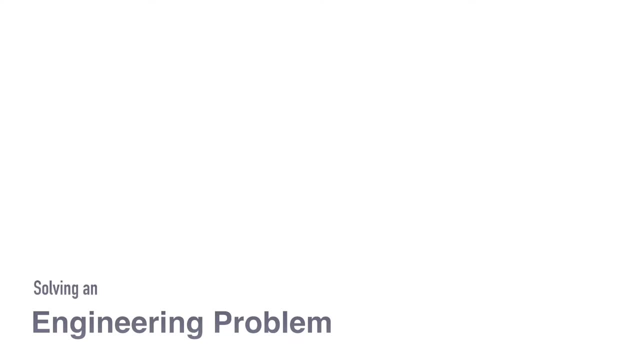 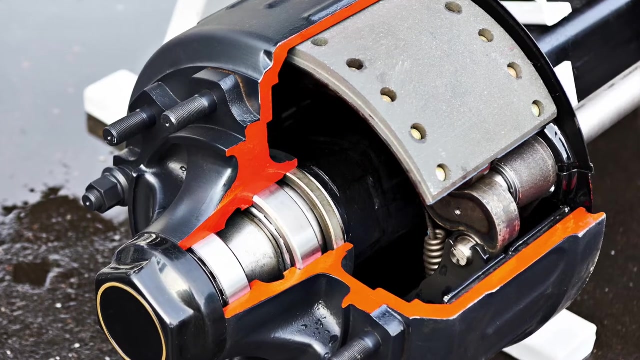 phases that are involved in solving engineering problem. So in CAE phase we are going to solve a engineering problem. Might be any problem. might be related to material, might be related to various characteristics And decision-making is available afterert. be related to cross-sectional area. might be related to thickness. might be related to total design. 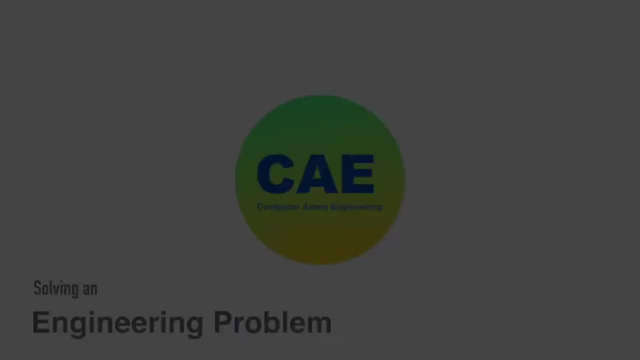 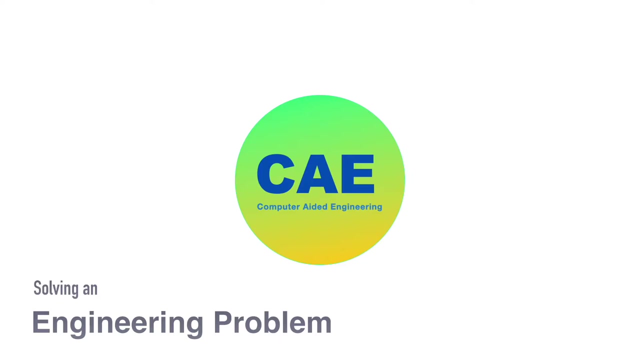 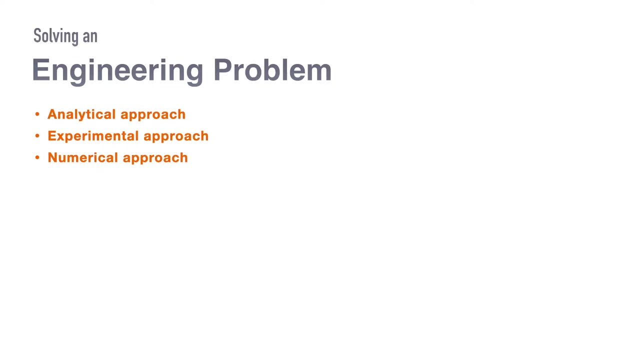 change. it might be anything. we will call it as in an industry, we will call it as solving an engineering problem in cae process. so to solve an engineering problem, again there are three approaches. first approach is analytical approach, second approach is experimental approach and third approach is numerical approach. so we'll discuss through these three approaches how we are going. 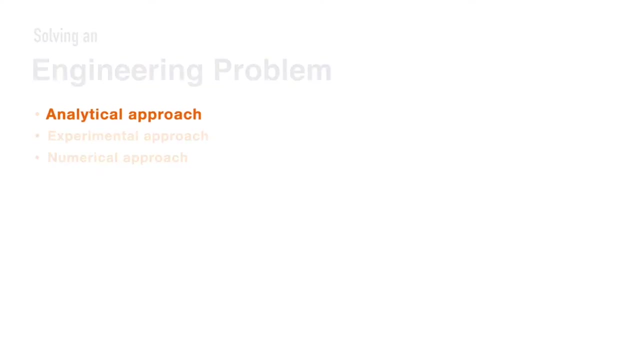 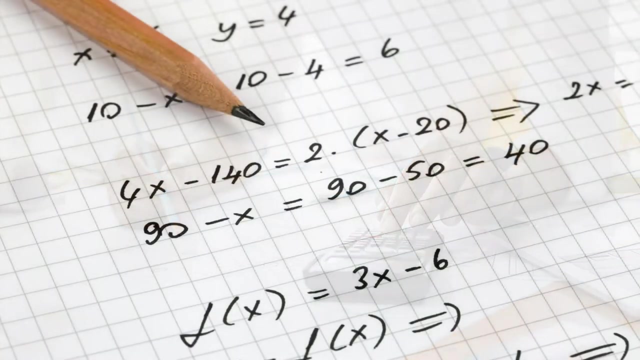 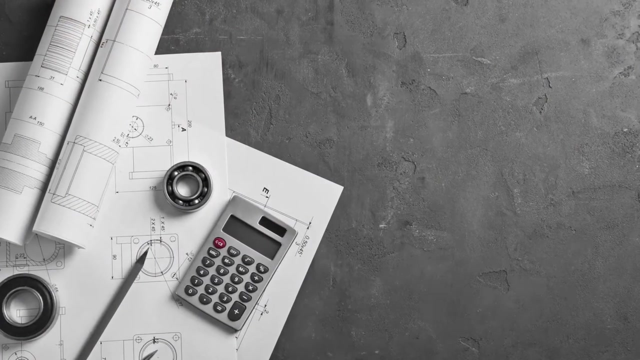 to solve an engineering problem in analytical approach. it is very familiar approach, everyone knows it. it is totally based on hand calculations. for this approach, we need equations. without that equations we are not going to solve that. and if you take an example, like i have a rectangle now i need to calculate an area. 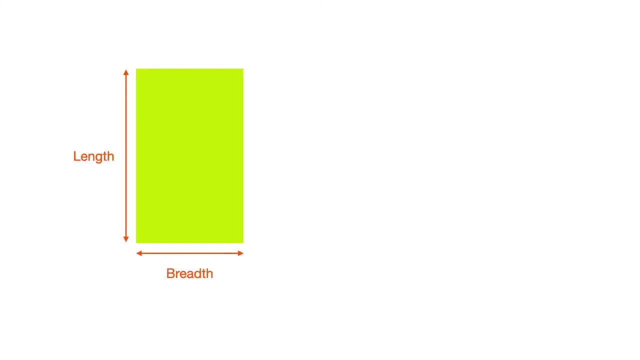 of rectangle, so i'll calculate it because i know length and breadth. i'll do that. i have a beam, a simple standard section, beam i section. i have a rectangle section, any section that should be a standard one. if i want to calculate moment of inertia, i will calculate because i have a ready. 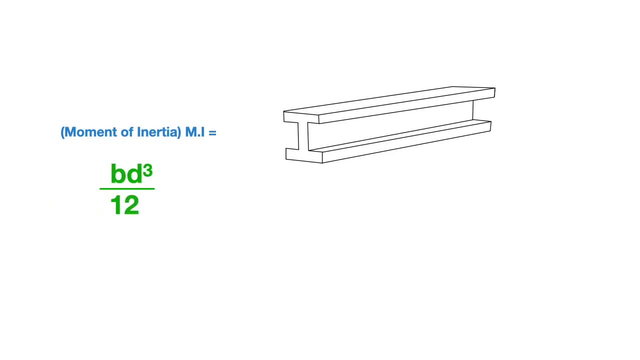 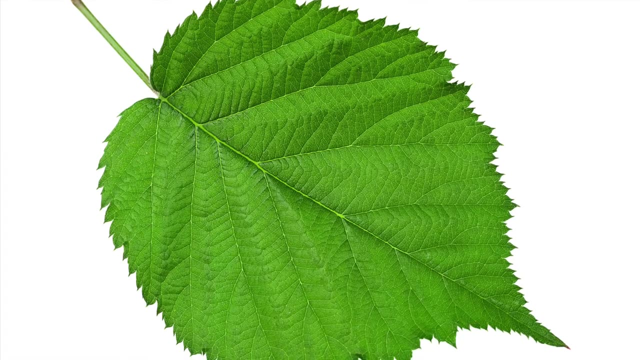 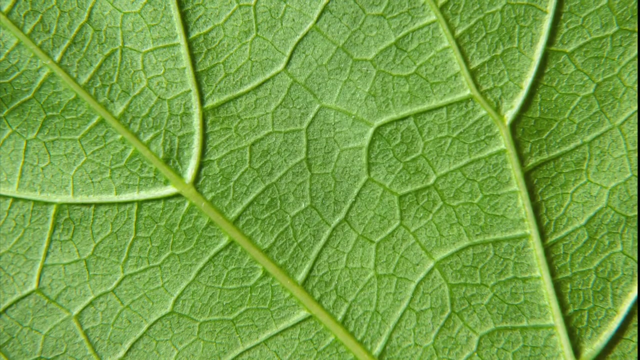 mode equation for that bd cube by dual. i have. so i'll do that. i'll get a solution. but take a leaf. we need to calculate area for leaf. so what i need to do? i need to divide the leaf into various sections, some rectangular sections and triangular sections. then i have to integrate it. 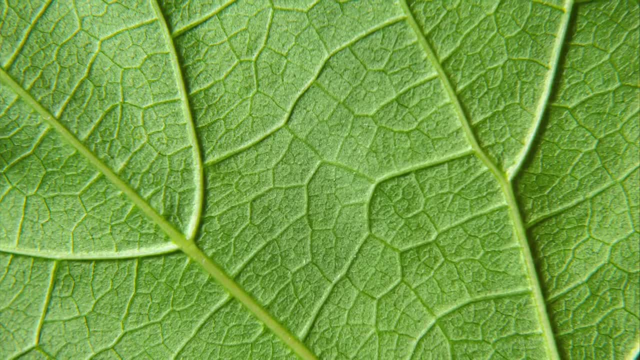 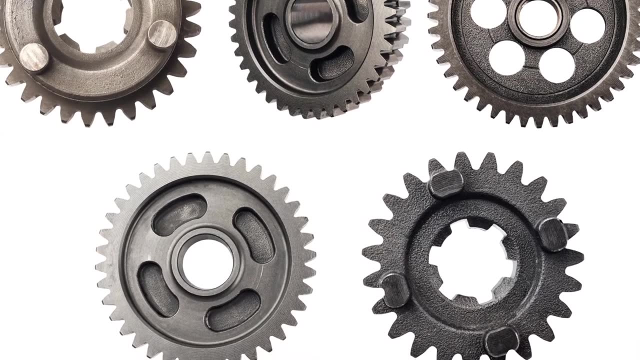 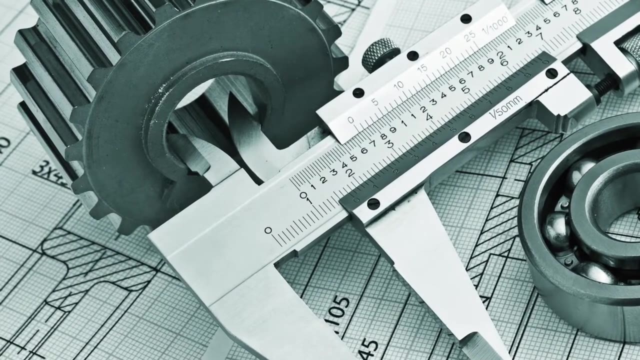 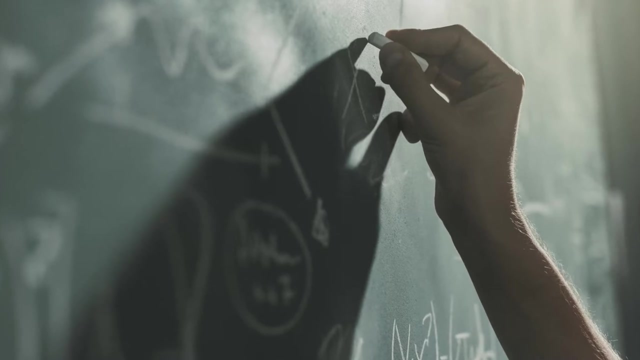 then i need to calculate, then come to a solution. if i need a moment of inertia for unstandard section, then what is the process? for me, readymade equation is not available, hence getting to the solution part is difficult. so generally this approach, the analytical approach, is called as: 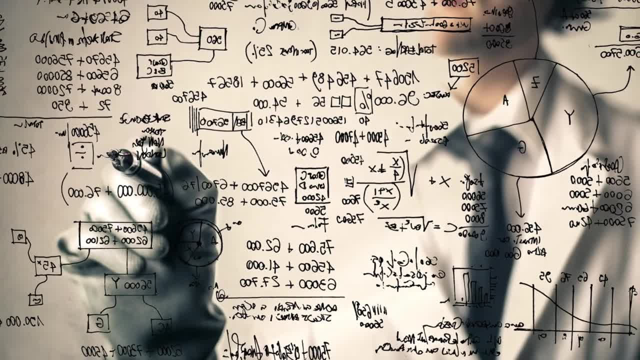 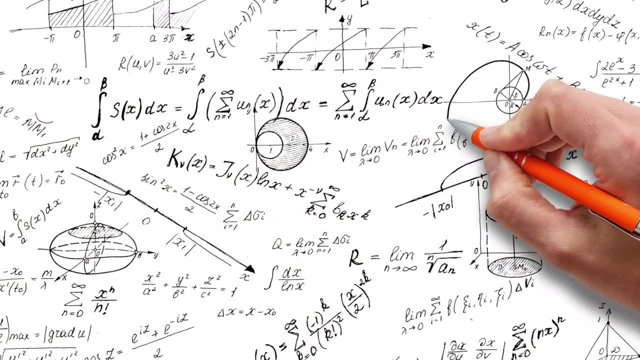 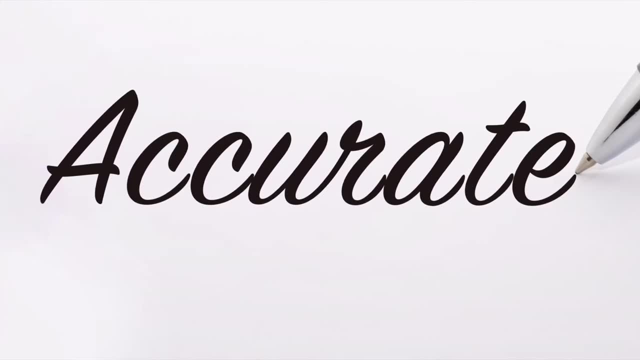 are known as scientists approach or scientists way of solving a problem. hence, if we look out the advantage of this approach, it gives us 100% accurate results, totally close to form. you can call it as a close to form- close to solutions we'll get. but there are major disadvantages of this approach also. 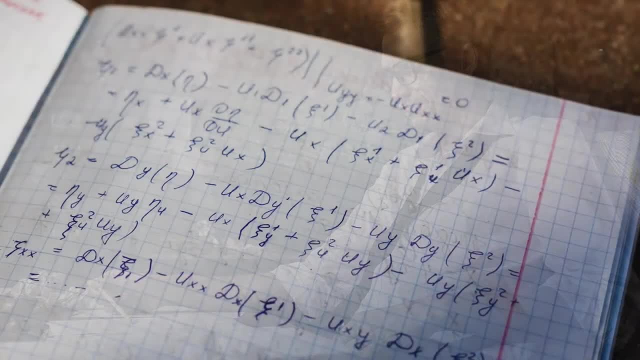 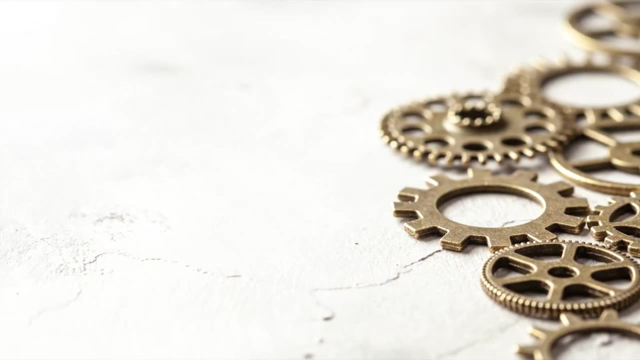 as we have discussed now itself. if i want an area of leaf, it is going to be difficult for me. if i want a moment of inertia for an unstandard section, then again it is going to be difficult for me. so in through this approach. if you want to solve an engineering problem, you can't solve all. 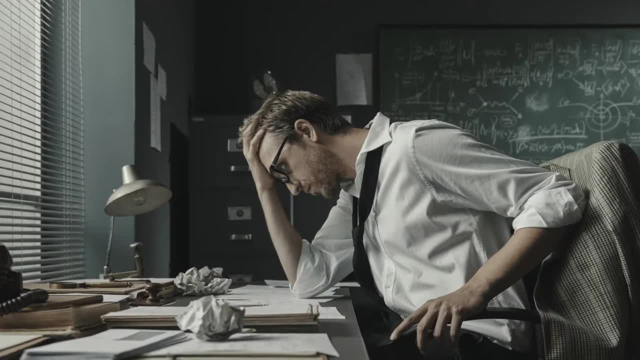 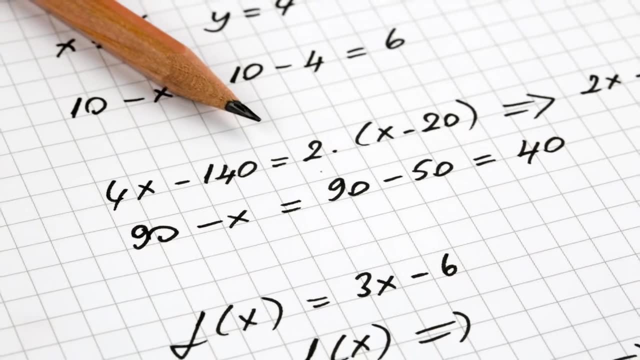 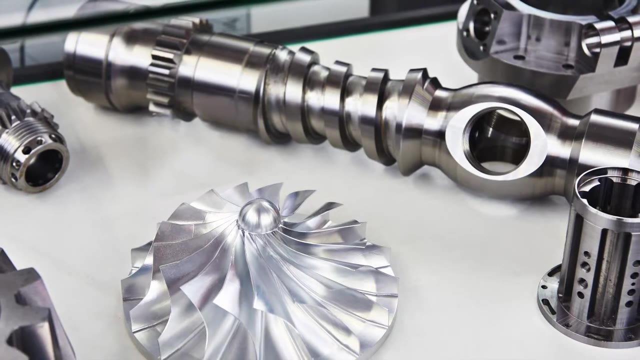 engineering problems. you can solve only those engineering problems where there are ready-made equations. ready-made equations are available, then you can solve it. otherwise you can't solve. consider about boundary conditions also. if boundary conditions are very simple, then you can solve this problem. if boundary conditions are very complex- I am related, environmental oriented- then 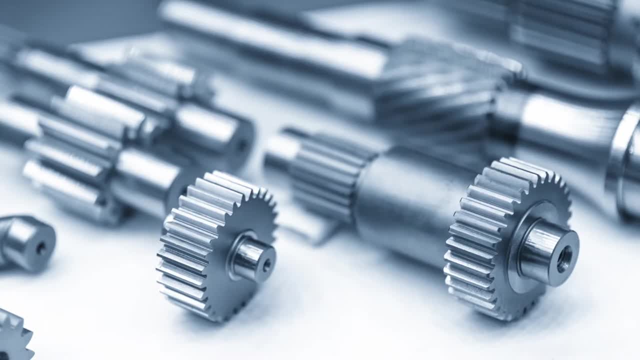 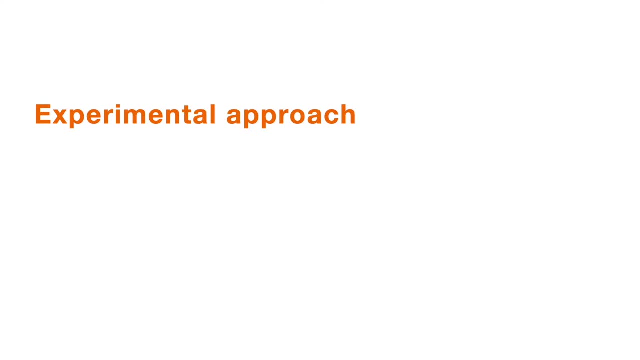 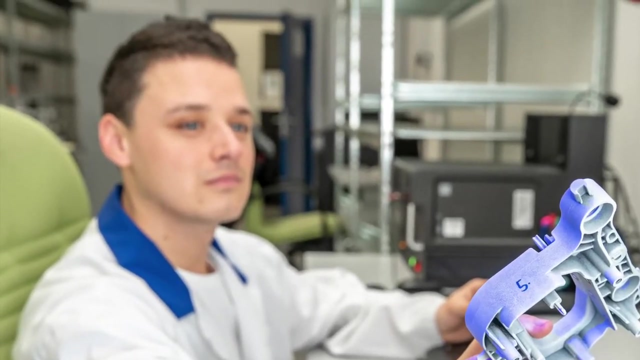 it is going to be difficult for us to solve. so let us move to the second approach: experimental approach. so in this approach, as it is experimental approach, we need prototypes. prototypes should be manufactured. at least three to five prototypes is needed. then again, we need to test those prototypes in order. 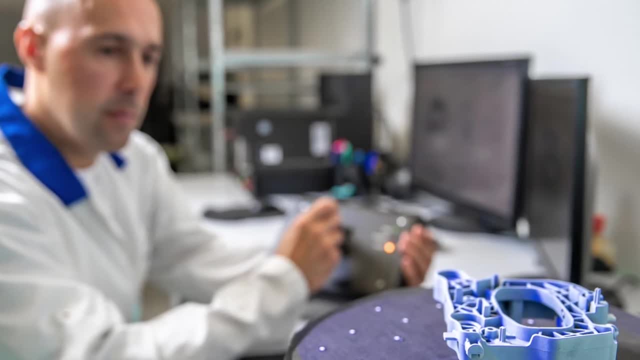 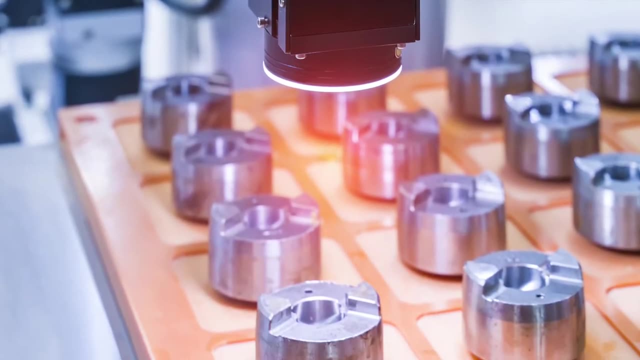 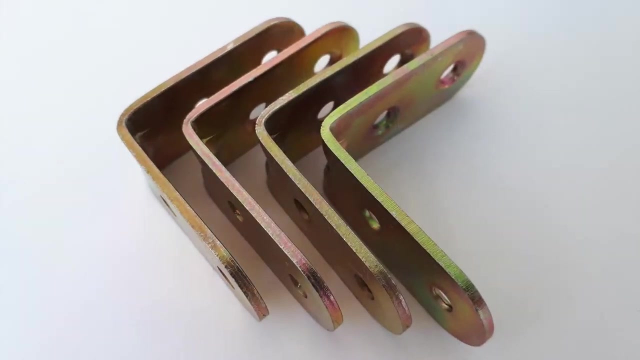 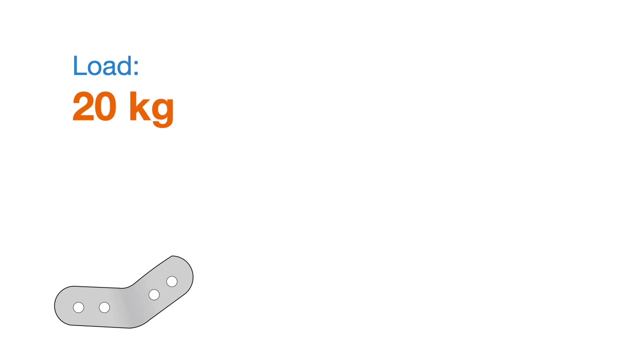 to test those prototypes, we need testing equipments, strain gauges, sensors, all those are required. so let us take an example here. so consider: a client is there, his requirement is to design a bracket which will take a weight of, or take a load of, 20 kgs, and he needs a factor of safety 1.5. so now you need 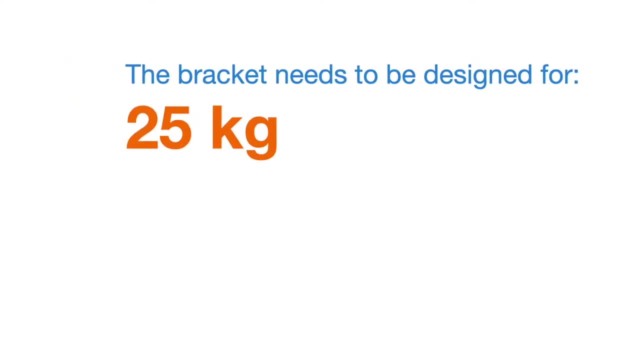 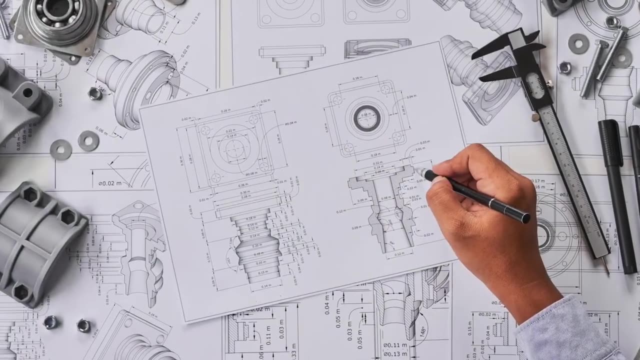 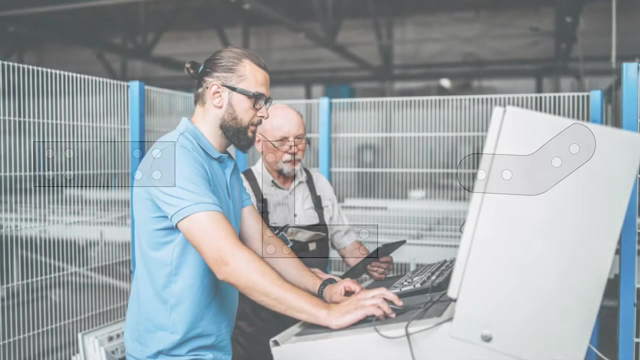 to design a design engineer to design it for 25 kgs. this is a requirement of client. design engineer will sit, he'll think about it. then consider he has proposed some design: a rectangle, a L shape, a bracket. so this should be manufactured again. they should be tested. so in testing, 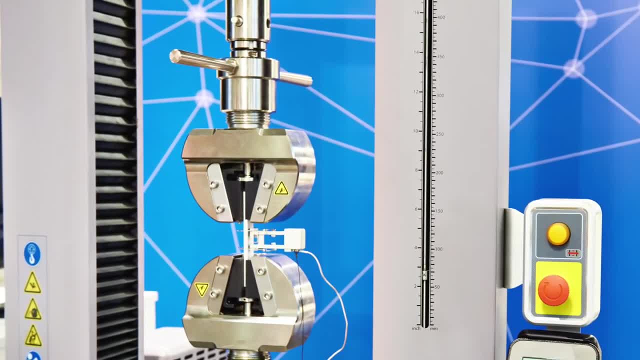 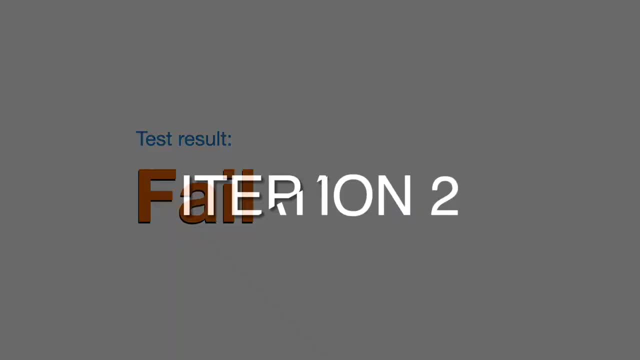 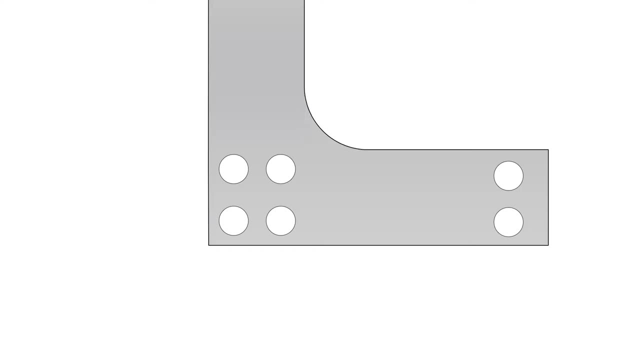 while testing. our testing in it came to a result that it is going to fail. it cannot take a load of 20 kgs. so again, iteration to in second iteration, design. you will sit and think, ok, let us add some fillet over the shop corner again. 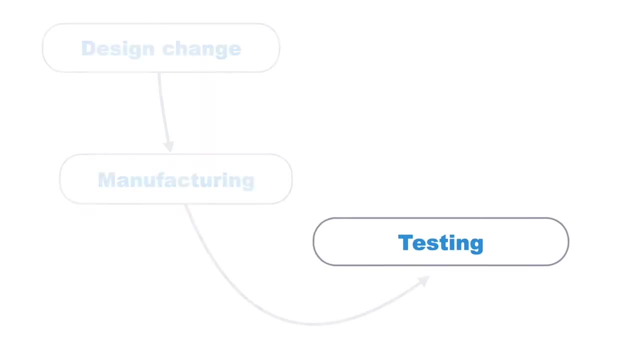 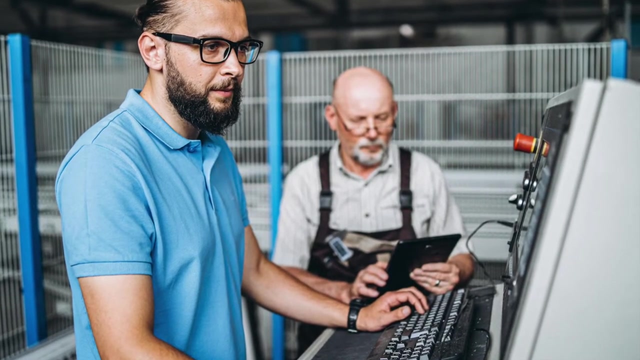 manufacturing. again, test in testing test engineer came to a conclusion. this test engineer came to a conclusion that the results is that it will take a load of 20 kgs, and that this engineer came to a conclusion that it is taking 20 kgs load but it is not able to satisfy the. 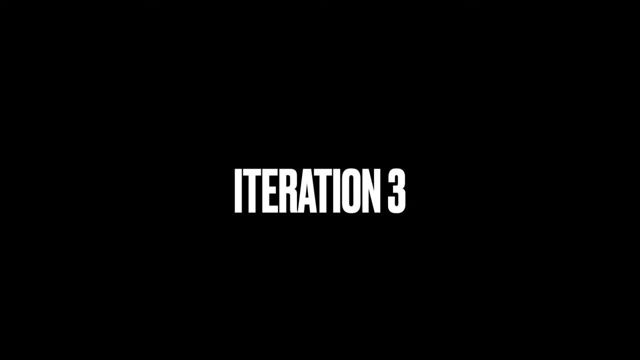 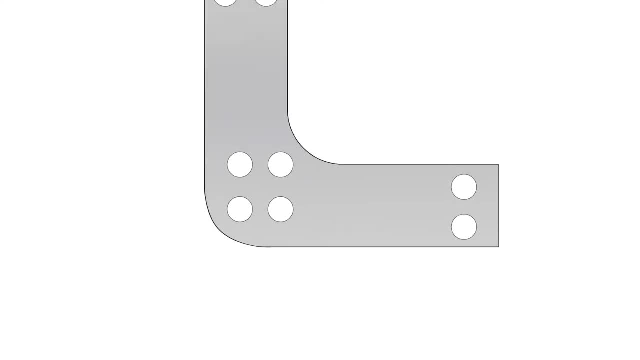 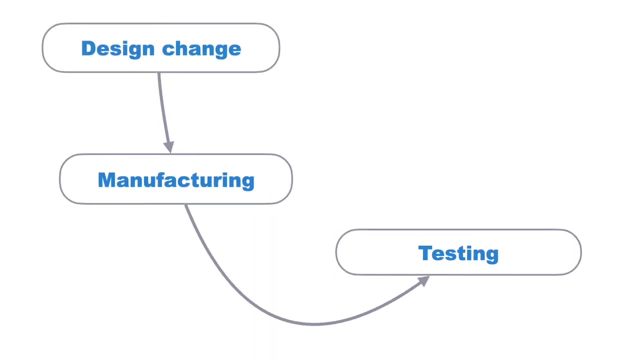 condition of factor of safety. so hence again iteration 3: design engineer will sit and again think. now he came to a idea that let us add a fillet, let us add a stiffener or rib to a bracket. again manufacturing, again testing. so in this testing test, engineer came to our conclusion that 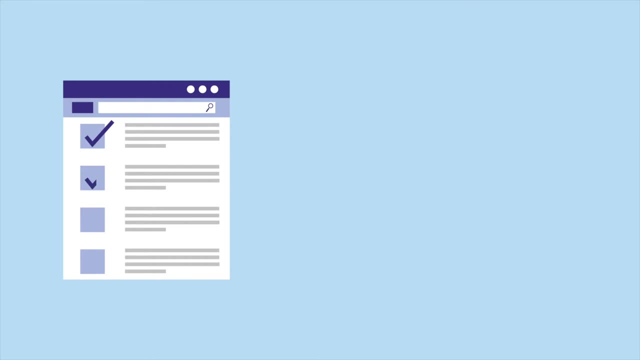 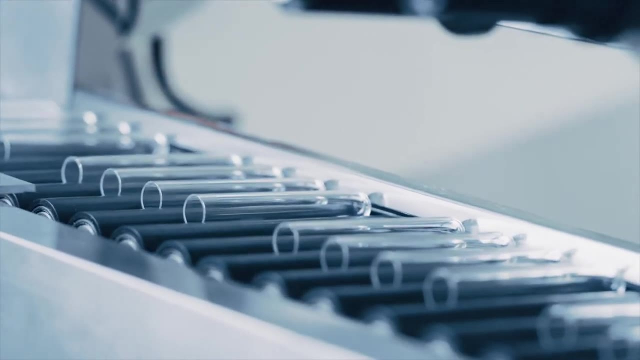 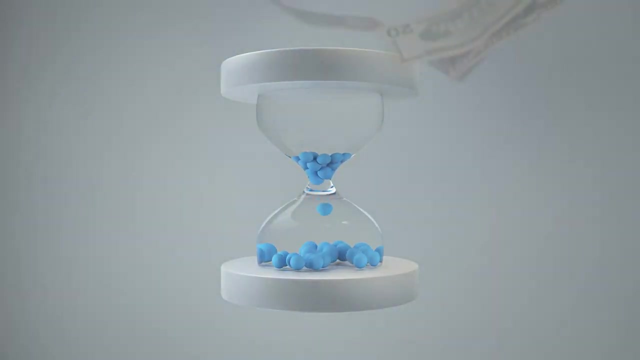 it is satisfactorily achieving all the conditions. hence this is a final design. it is approved design. now it will. this design will be taken for mass manufacture. so hence, if you see the process, throughout process, it is a time-taking process as well as money involved process. it's a simple. 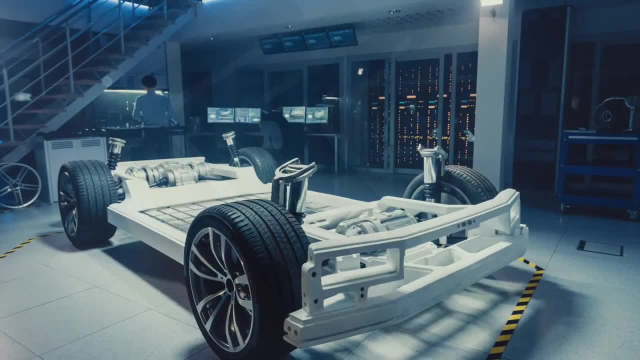 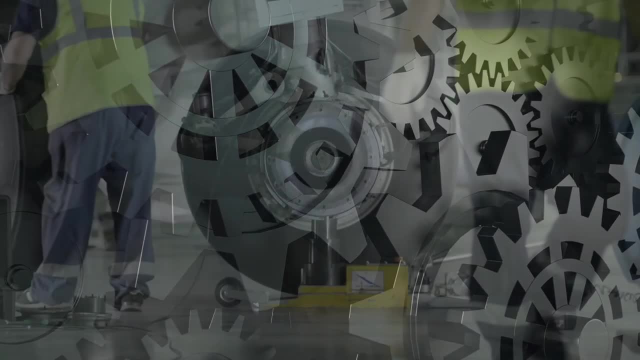 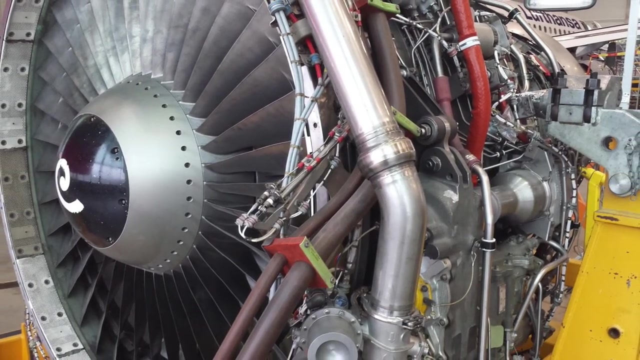 bracket. you can do it within half day or one day. but think about a car, think about a heavy machinery, think about aero components, think about automobile components, think about marine components. you can't do that, okay. you cannot just manufacture a car, crash it, okay. so you came to conclusion that 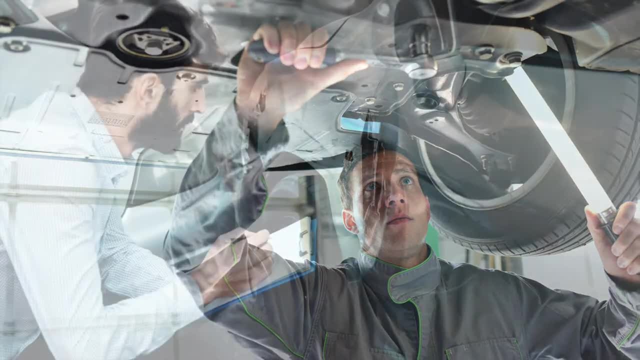 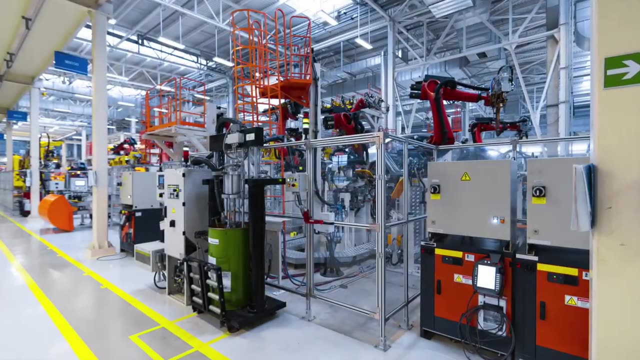 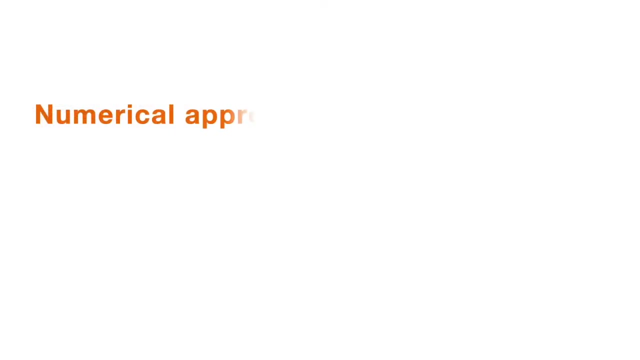 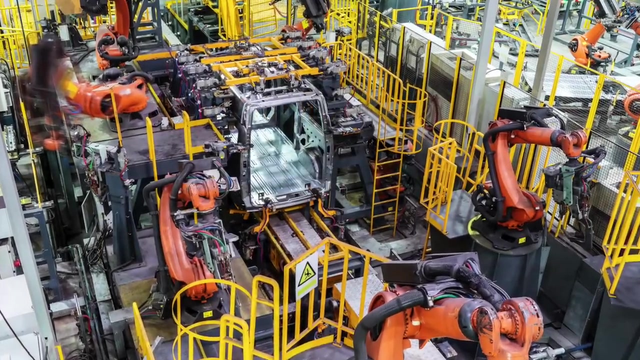 is not satisfying. again manufacture one more car, again crash it, so you cannot go. iteration process. it is time taking process as well as money involved process. so the industries, whatever industries are there, they are focused or devoted towards numerical approach. hence numerical approach has gained a lot of market over the industries. now let us discuss about a 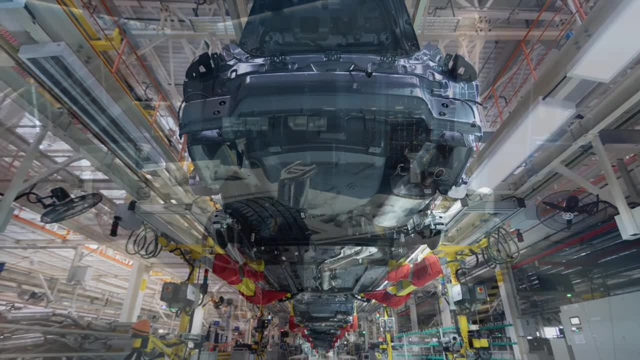 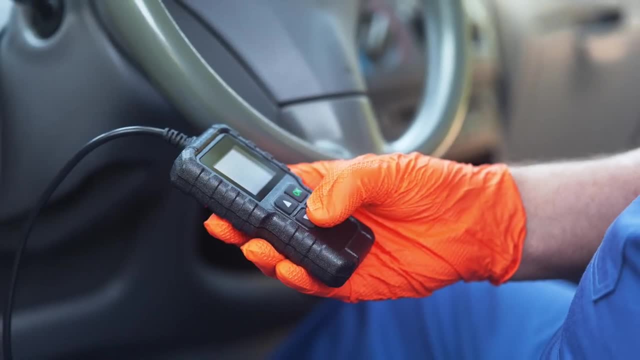 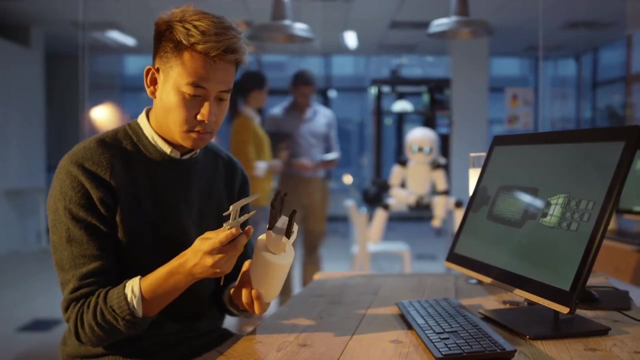 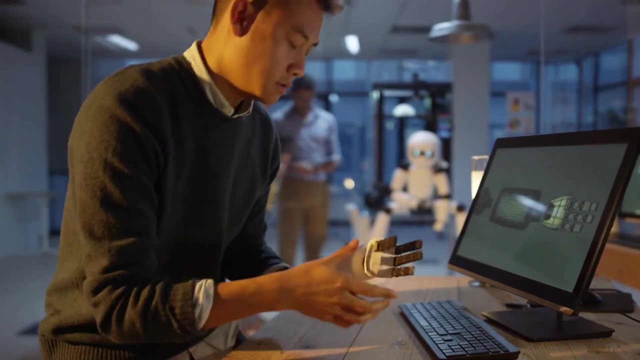 numerical approach. in numerical approach you no need any prototypes, no need any testing equipments, no need of any basic formulas, ready-made equations. only you need a experienced engineer and a good configuration system. so all difficult process. you need a good configuration system. so all difficult problems related to any boundary condition problem and you can do iterations many times we can change.